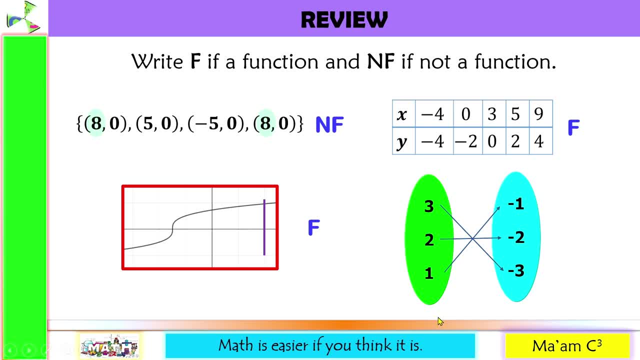 For the last one, we have a map, and let us examine this. All values of x are mapped to a number in the second group, and each x value here is mapped to only one value in the second group. So therefore, this is a function. Now I am going to teach you to determine if an equation is a function or not. 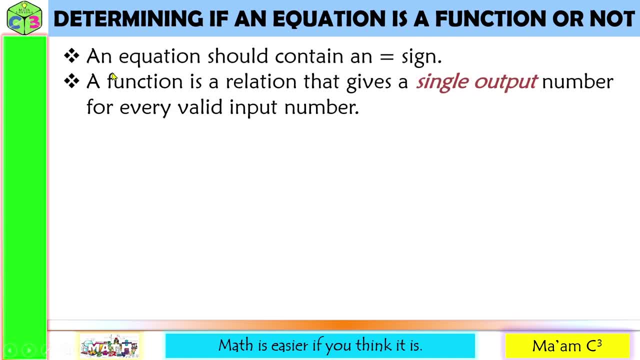 You have to consider two things. One, an equation should contain an equal sign. We cannot call it an equation if it does not have an equal sign. And second, remember the definition of a function. It is a relation that gives a single output number for every valid equation. 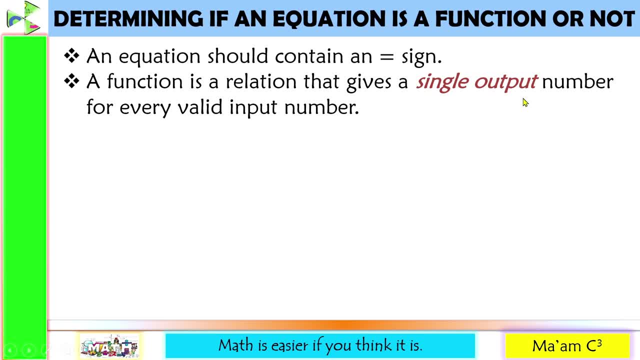 Input number. So this means in any given equation we need to solve the equation for y and analyze if there are any values of x that can be substituted to the equation that will give different values of y. If there is only a single output of y for every value of x, then the equation is a function. 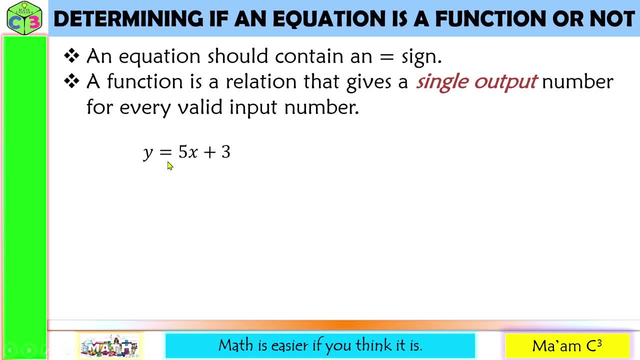 Let us have an example. You will notice here that we have an equal sign and since this is a relation, we should have two variables: the independent and the dependent variables, the x and y. Now let us examine if this is a function or not. Think of a value that you can substitute for x and analyze if it will. 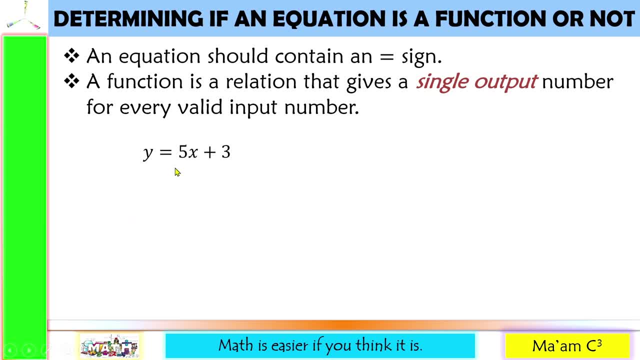 give you a single output for y. Let us try zero. Five times zero is zero and zero plus three is three. So if your x is zero, your y is three. Let us put that in a table. Let's try another value. 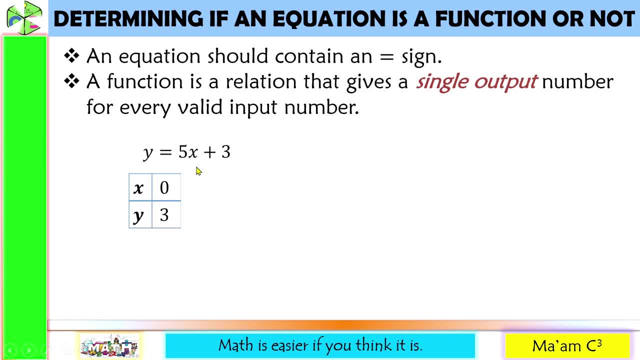 Let us say positive one Five times one is five and five plus three is eight. So if your x is one, your y is eight. Let's have another one. Let us say negative one Five times negative one is negative five and negative five plus three is negative two. Notice that for every unique value. 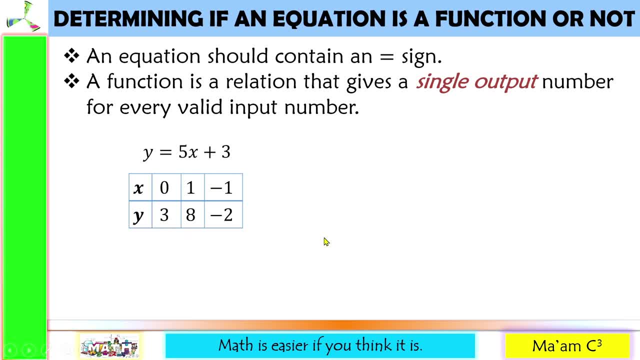 of x, we have a single output for y. Therefore, this equation is a function. Let's have another one: x squared is equal to y plus one. Let us isolate y, So let us move one on this side. This will become: y is equal to x squared minus one. So our y is already defined and we do not have 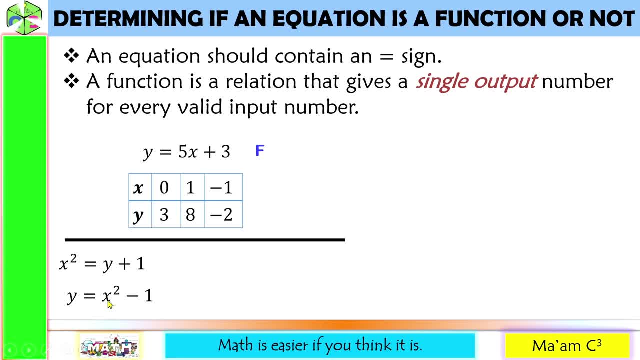 any more y's. here on the right side We have an equal sign and we have two variables. Now let us look at the x values Again. let us start with zero. Zero is squared is zero, and zero minus one is negative one. So if your x is zero, your y is negative one. Let us try positive one. One is: 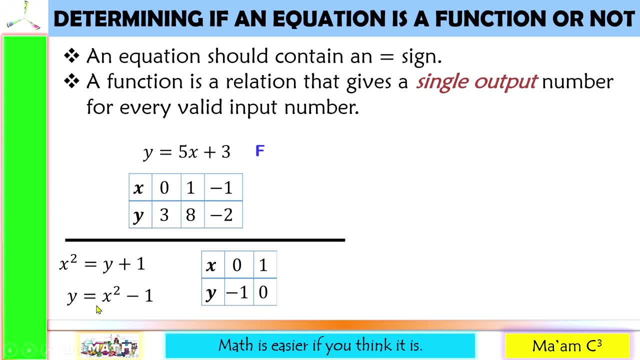 squared is one and one minus one is zero. Let's have negative one. Negative one is squared is one and one minus one is also zero. Remember what you have learned in table of values, We simply take a look at the x values and there should be a negative one. So let's try positive one. Let's. 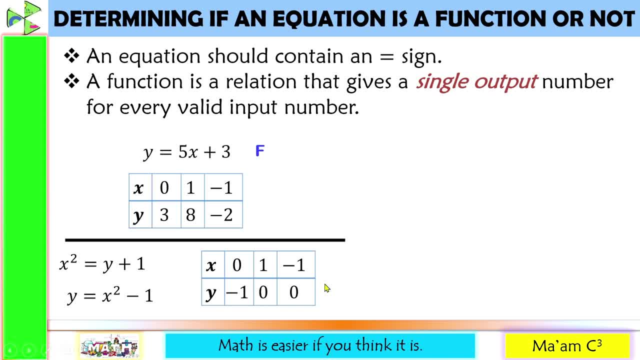 have another one. Let us isolate y and make it positive, So this will become two. y is equal to x squared minus seven. To solve for y, we're going to divide both sides by two. Two and two here will cancel out, leaving us y, And on this side we have x squared minus seven. all over two We have. 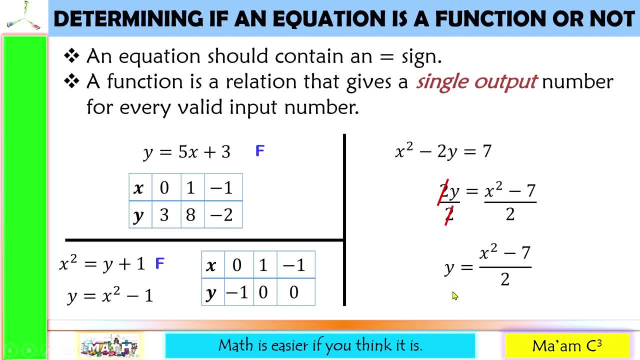 an equal sign and we have a negative one. So let us isolate y and make it positive. So this will have x and y. Our y is already defined. We do not have any more y's on the right side And when you substitute any number for x, if you have trouble thinking what numbers to substitute, use our. 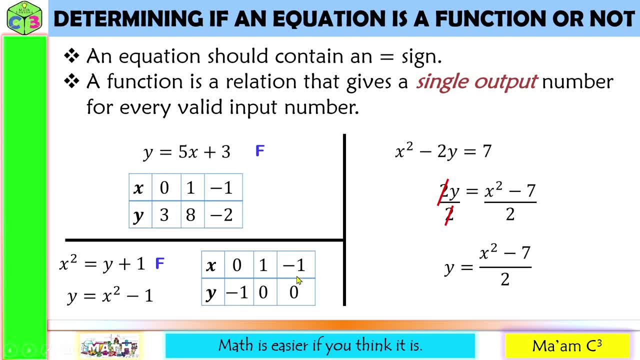 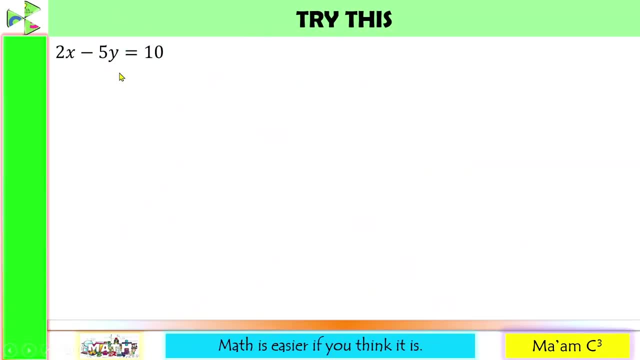 technique here. Substitute zero positive number and negative number And you will see that for every unique value of x you will get a unique value of y. Therefore this equation is a function. Try this: Two x minus five y is equal to ten. Let us isolate y and make it positive, So this will become five y. 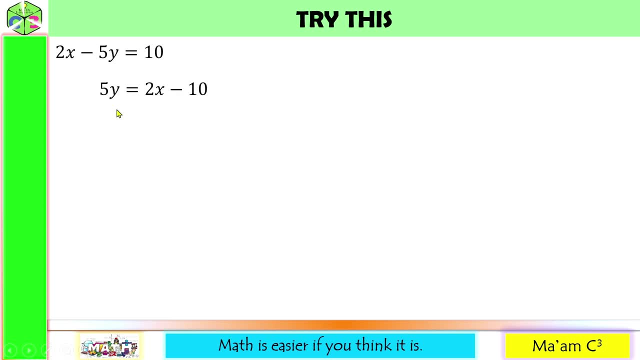 is equal to two x minus ten. To solve for y, let us divide both sides by five. Five and five here will cancel out, leaving us y. Then we have here two over five of x, And then ten divided by five is two. We have an equal sign. We have x and y And our y is already defined. We do not have any. 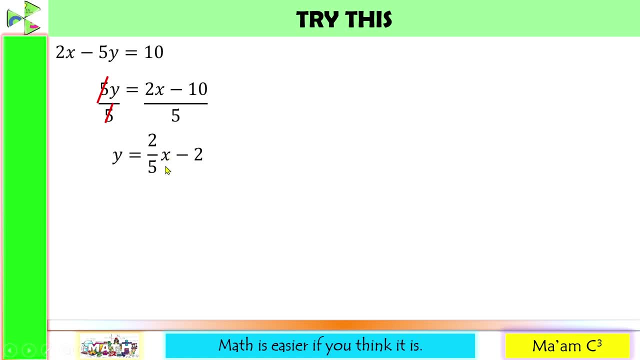 more y's on the right side. So let us solve for y, And then we have two over five of x, And then we have two over five of y's on the right side, And if you substitute any value for x, you will get. 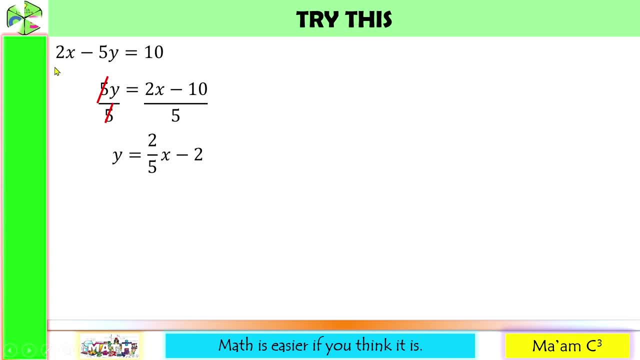 a unique value of y. Therefore, this equation is a function. Let us have another one. We have x squared plus y squared is equal to 100.. We have here an equal sign And we have x and y. For some of you, you will notice that this equation is an equation for a circle And using a vertical line. 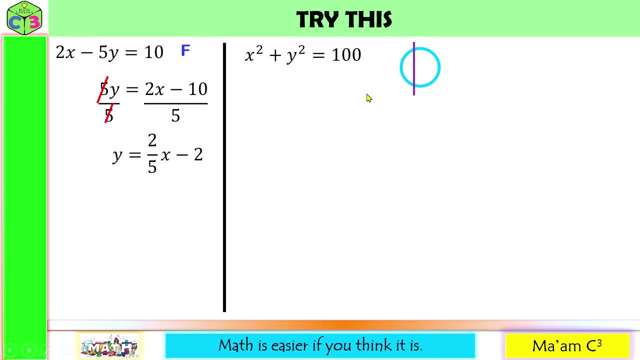 test. we know that a circle is not a function. But what if you do not know the graph of the equation? So let us isolate y here. Let us move x squared. on this side We have: y squared is equal to 100 minus x squared. To solve for y we have to take the square roots of both sides, So this: 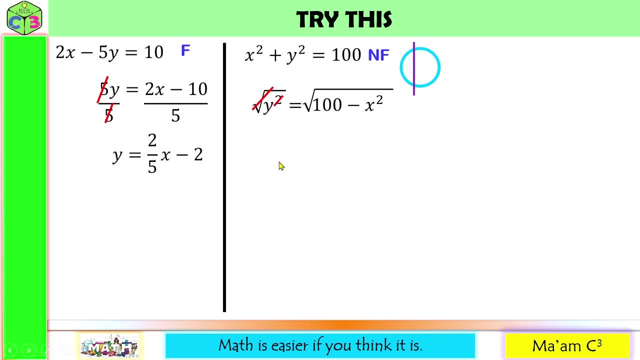 radical symbol and this exponent will simply cancel out And the square root of the right side will give two answers: positive and negative. Let us make this simpler. For instance, you have y. squared is equal to 100.. To solve for the value of y, you are going to take the square roots of both sides. 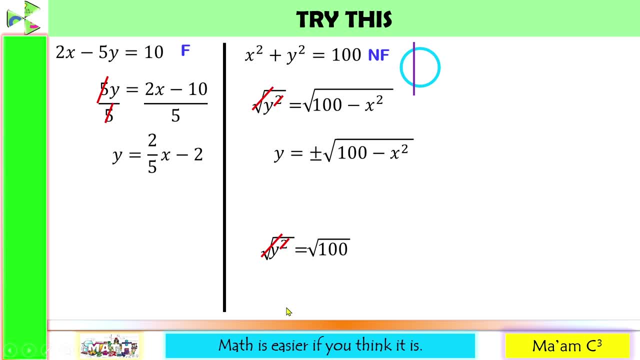 So this radical symbol and exponent will simply cancel out. Now the square root of 100 will give you two answers. Those are positive and negative 10.. Positive 10 squared is 100. Negative 10 squared is also 100. So when you take the square root of 100, it gives you two answers: positive and 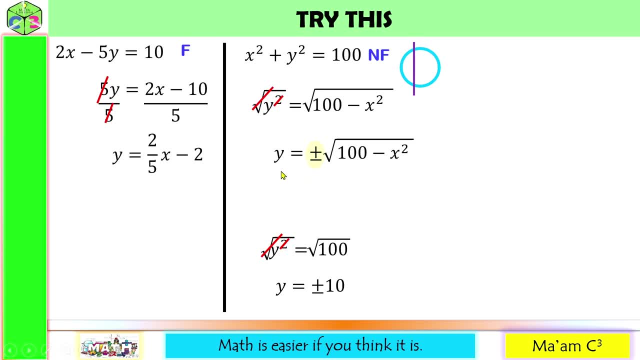 negative. That makes our y not unique. That is why this is not a function. Let us have another one. This time we have y. cubed is equal to x plus 3. To solve for y we have to take the cube root. 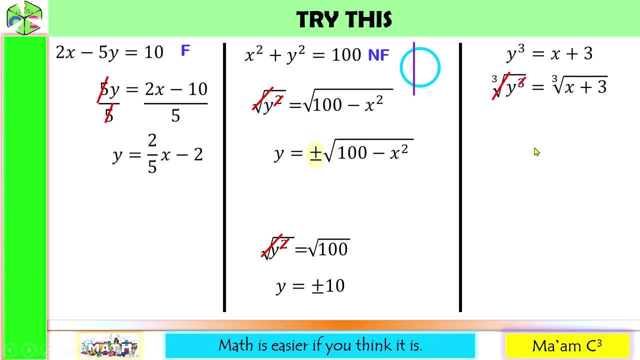 of both sides. So this will cancel out. So we have: y is equal to cube root of x plus 3.. Let us make this simpler here. like this one. Let us say you have y, cubed is equal to 27.. To solve for y you take the cube root of both sides. 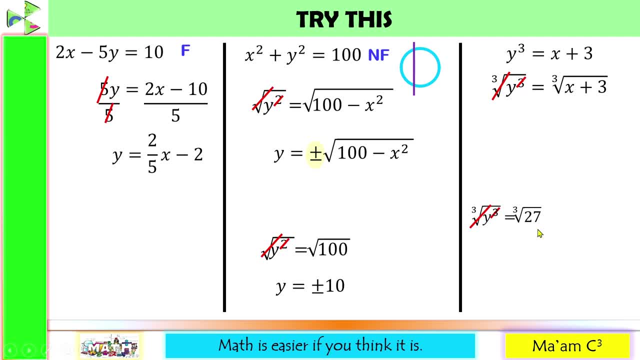 So this will cancel out And the cube root of 27 is positive 3.. If you have y, cubed is equal to negative 27, taking the cube root of both sides. so this will become y And the cube root of negative. 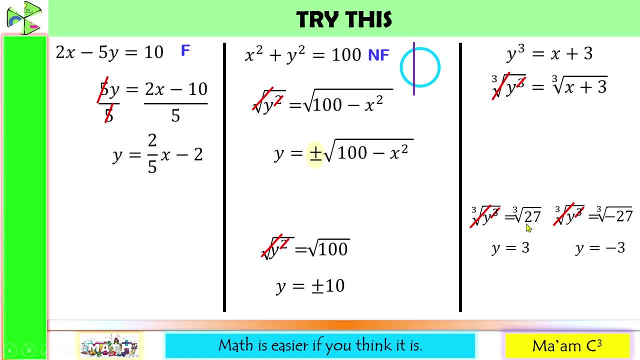 3.. The thing here is every number gives a unique cube root. If your number is positive, it will give you a positive cube root. If your number is negative, it will give you a negative cube root. So your y here is defined. The cube root of x plus 3 will give you a unique value of y. Therefore, 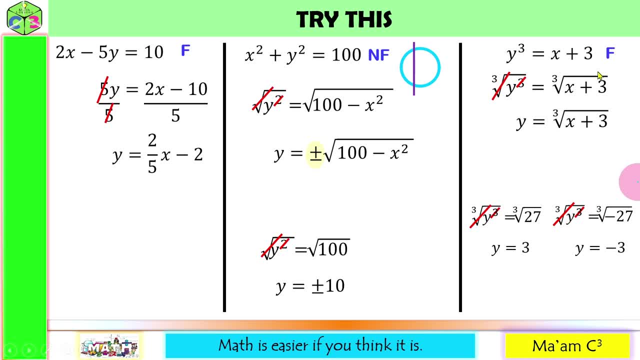 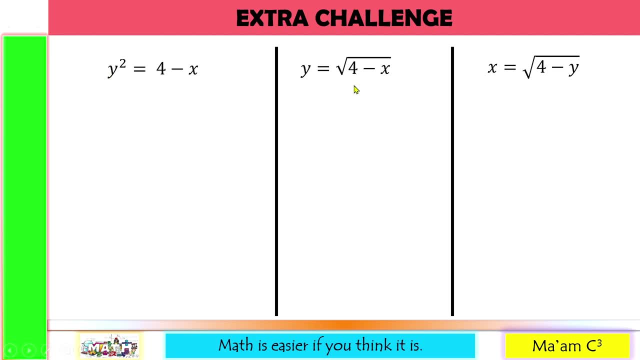 this equation is a function. Let us do extra challenge For each of the equation. here we have an equal sign and we have x and y. Now let us analyze each one of them. For this one, to solve for y, you have to take the square roots of both sides. 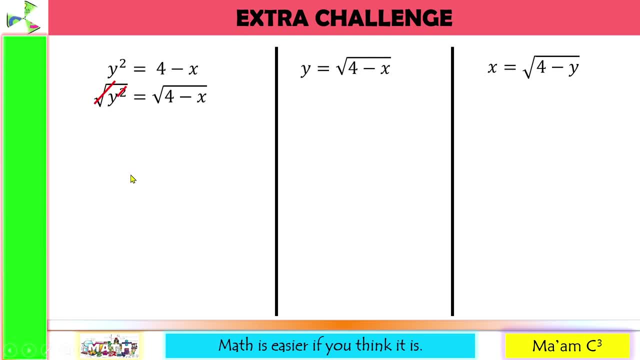 So the radical symbol and the exponent will simply cancel out. And since you take the square root of the right side, it will give you two answers, positive and negative. And since you have two answers, that means your y is equal to negative. So you have to take the square root of both sides. 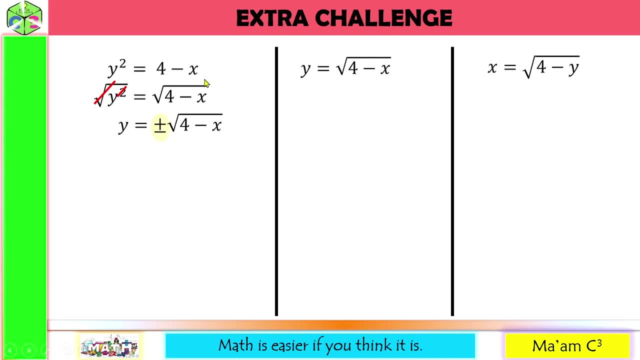 Therefore, this equation is not a function. For this one we have, y is equal to the square root of 4 minus x. The difference of this equation from here is that in here you take the square root of both sides, While on this one your y is already defined. This means you are only asked to get the 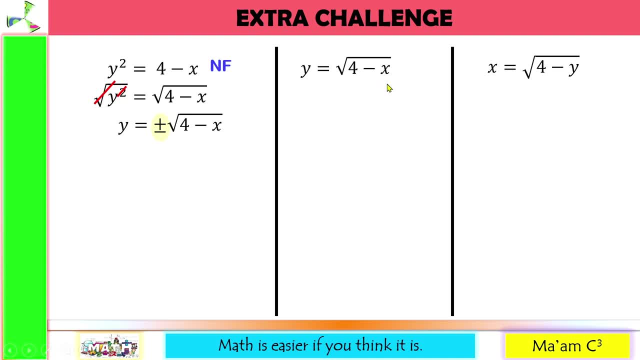 positive root of 4 minus x. Therefore, this equation is not a function. For this one you have, y is equal to the square root of 4 minus x. If you have here a negative symbol, then it means you are asked to give the negative root of 4 minus x. 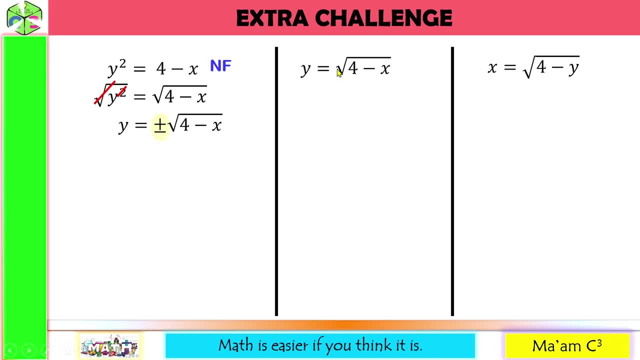 So, whichever is the case, positive or negative root, your y is unique. You only have one value. Therefore, this equation is a function. Now for this one. the only difference of this equation to this one is the placement of the variables. Here I have y, here I have x, Inside the radical. 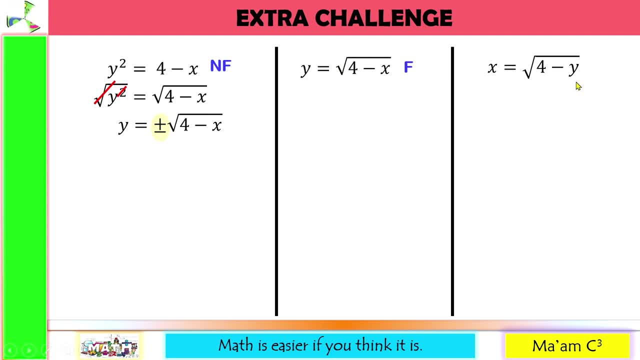 symbol here is x. here I have y To solve for y. we are going to square both sides, The radical symbol here and the exponent will cancel out. So we have x squared is equal to 4 minus y. Let us isolate y and make it positive. So we have y is equal to 4 minus x squared. Now our y is defined. 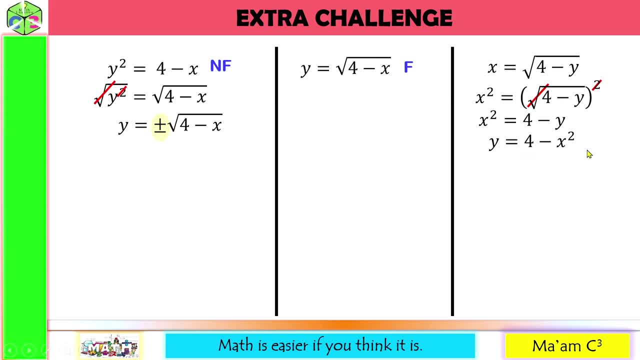 We do not have any more y's on the right side of the equation, And when you substitute any value for x here, you will get a single output for y. Therefore, this equation is a function. I still have some space here. Let's have some more. 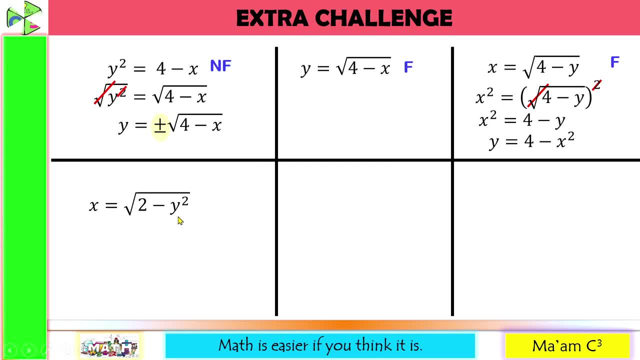 I have here an equal sign and also the x and y To solve for y, let us square both sides, So this radical symbol and this exponent will cancel out. So we have: x squared is equal to 2 minus y squared. Let us isolate y and make it positive. This will become: y squared is equal to 2 minus x squared. 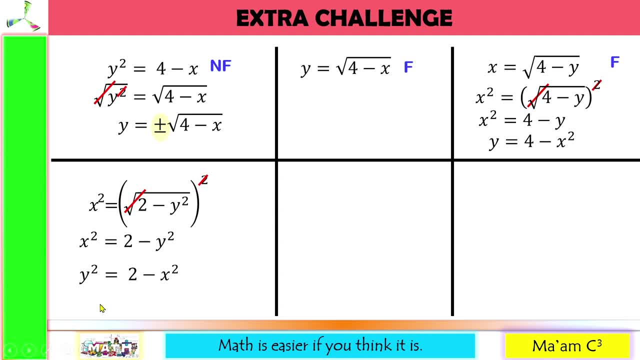 And to solve for y, we're going to extract the square roots of both sides. The radical symbol and the exponent will cancel out, And this will give us two answers, positive and negative. Since we have two answers, it means our y is not unique. Therefore, the equation is: 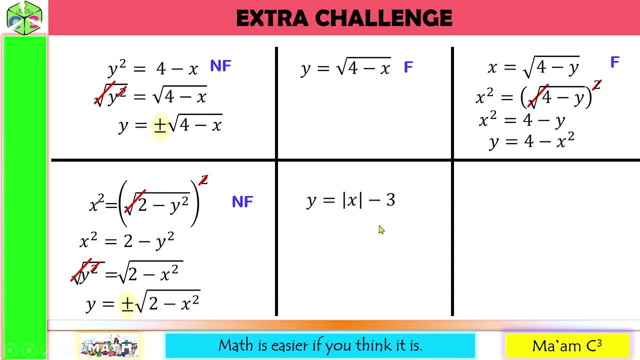 not a function. Let's have another one. Y is equal to the absolute value of x minus 3.. The absolute value function makes any value substituted here positive. Let us try: 1. The absolute value of 1 is 1 and 1 minus 3 is negative. 2. If we have negative 1, the absolute value. 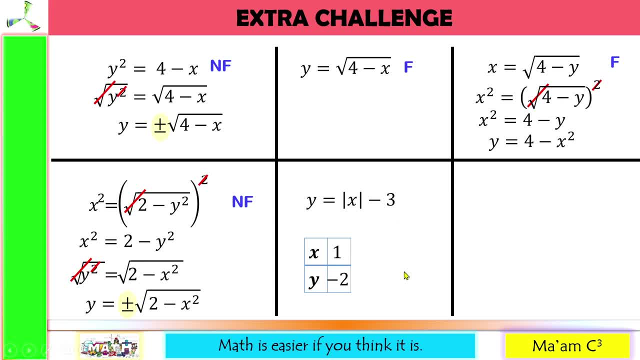 of negative. 1 is still 1 and 1 minus 3 is negative 2.. Again for the table of values, we are only concerned with the absolute value of x minus 3.. So we have 1 minus x squared and 1 minus 3 is negative 2. We are only concerned for the x values. No x value must. 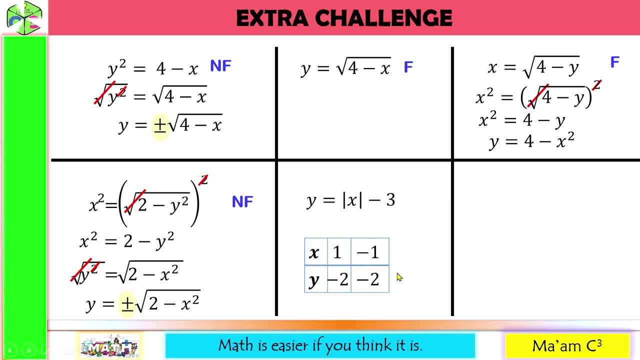 be repeated, And here there is none. Therefore, this equation is a function. Now let's have this one. This time y is inside the absolute value symbol. Let us recall the definition of absolute value: It is the distance of the number from 0. So let us say you have. 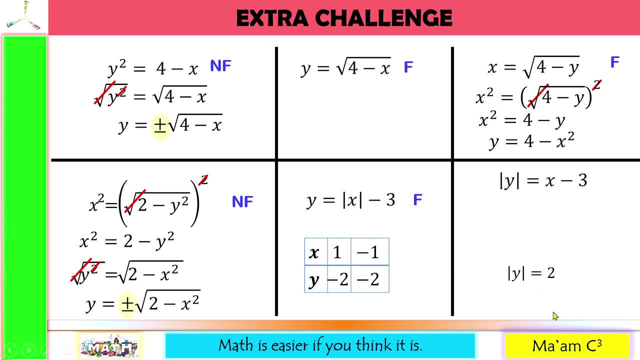 the absolute value of y is equal to 2.. Y here could be 2. Since the absolute value of y is 2.. Y could also be negative 2. Since the absolute value of negative 2 is also 2.. So this means: 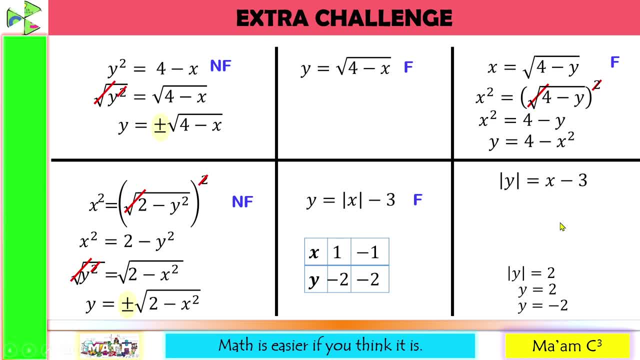 your y has two different values. So in this equation, y could be x minus 3 and y could be the opposite of this. This means when y is inside the absolute value symbol, it gives us two different answers. Therefore, this equation is a function. So let us recall the. 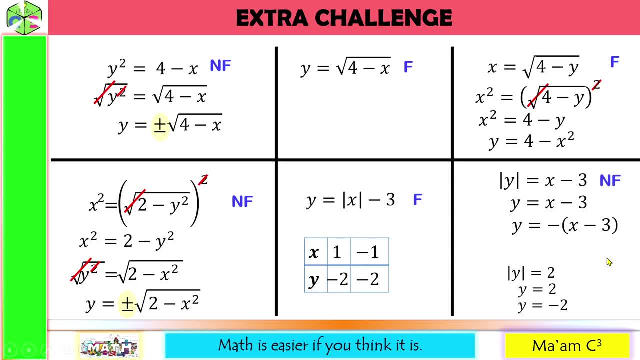 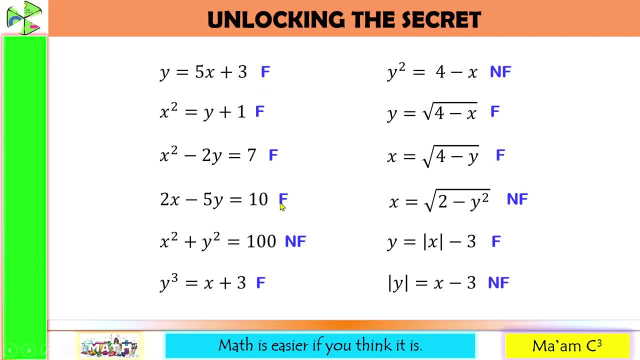 definition of absolute value symbol. This equation is not a function. Now let us unlock the secret. I have listed here all the equations that we discussed and if it is a function or not a function. Can you now tell me if an equation is a function or not a function? 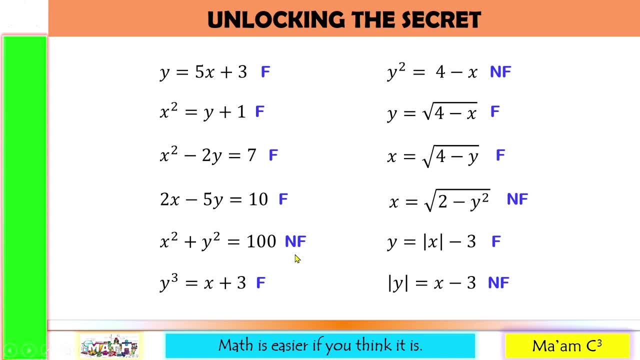 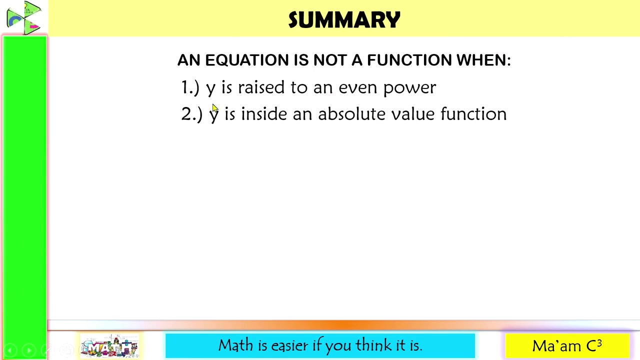 by simply looking at it. I'll give you a few seconds to think about it, or you may pause this video if you want more time, Let me now reveal the secret. An equation is not a function when y is raised to an even power or y is inside an absolute value function. Let's take a look back Here. the exponent: 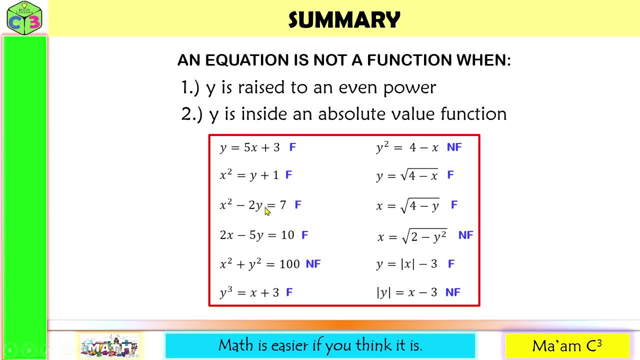 of y is 1.. Here it is also 1.. In here it is also 1.. And in here it is also 1.. And 1 is an add number. That's why these four equations are function. In here, the exponent of y is 2. And 2 is